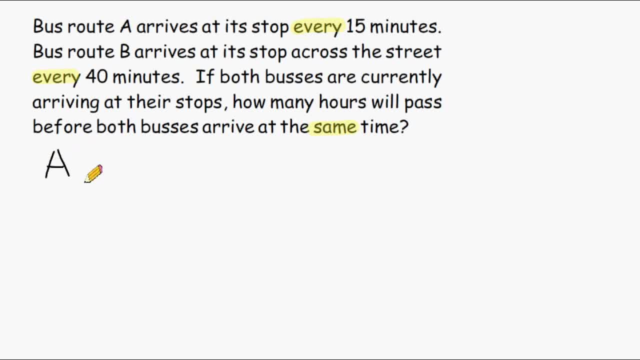 So right now, bus A and bus B are at the bus stop at the same time, across the street from each other. So both buses are leaving at the same time And we have to figure out how many more minutes left And we have to figure out how many more minutes later that both buses will be at the bus stop at the same time. 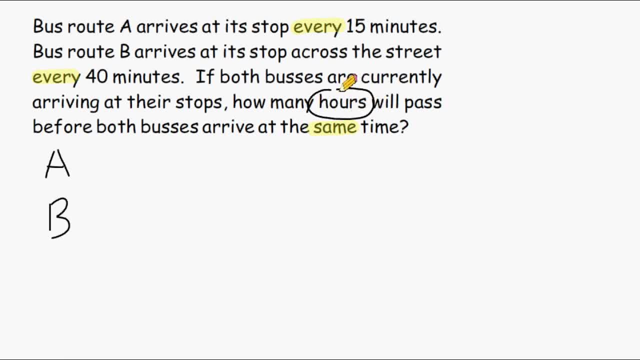 Actually the question reads how many hours will pass, not how many minutes. But notice in the problem, they give us minutes and the question asks for hours. So we have to keep that in mind when figuring out the answer. So, starting with bus route A, 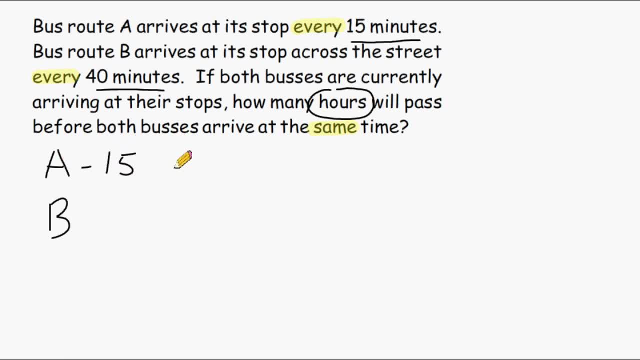 So bus route A is going to arrive 15 minutes later, And after that it would be 30 minutes later. Plus another 15 minutes would be 45 minutes, And then 60 minutes, Which is exactly one hour. Plus another 15 minutes would be 75.. 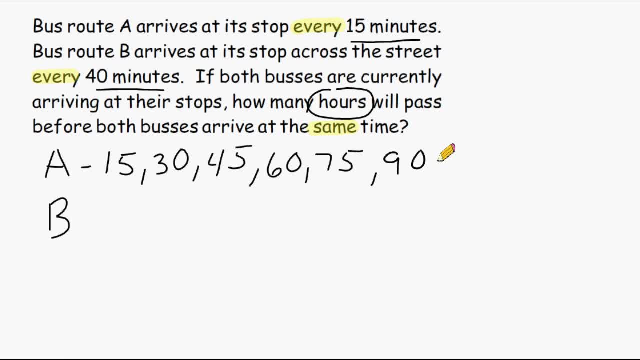 Another 15 minutes would be 90. Plus another 15 is 105 minutes, And another 15 minutes would be a total of 120.. Now let's take a look at bus route B. Now, bus route B does not run as often as bus route A. 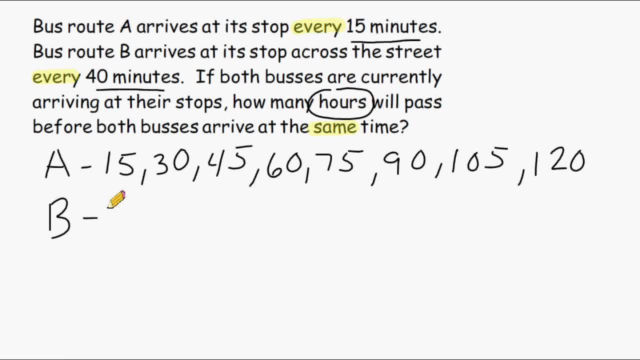 Bus route B arrives every 40 minutes, So another bus would come along 40 minutes later And then 80 minutes later, And then 120 minutes later, And at this point I'm going to stop, because we have a common multiple in both lists. 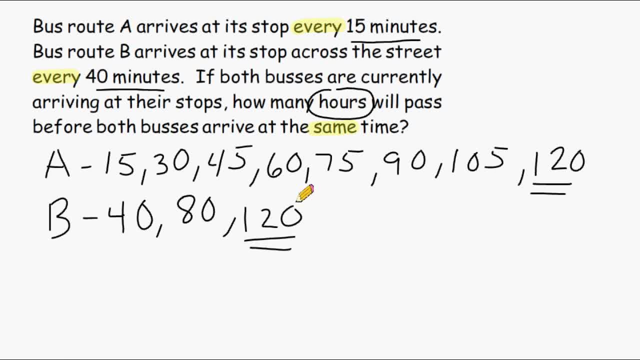 And that is our first common multiple. Now a lot of people are hasty to just circle that common multiple and think that that is their answer. But in this case it would not be the answer, Although both buses would arrive at the same bus stop 120 minutes later. 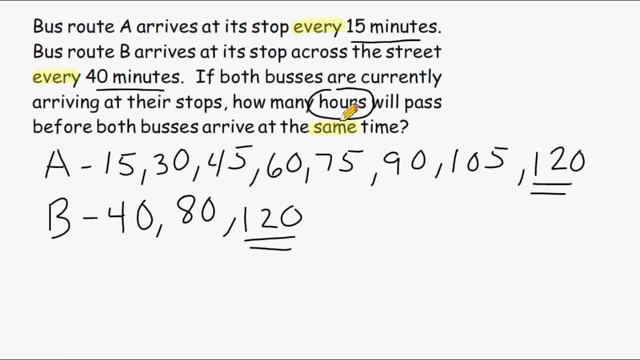 The question is specifically asking how many hours will pass, Because we know there are 60 minutes in one hour. We have to take 120 minutes and divide it by 60 minutes And of course 60 fits into 120 twice. So we would say that both buses would arrive at the same time two hours later. 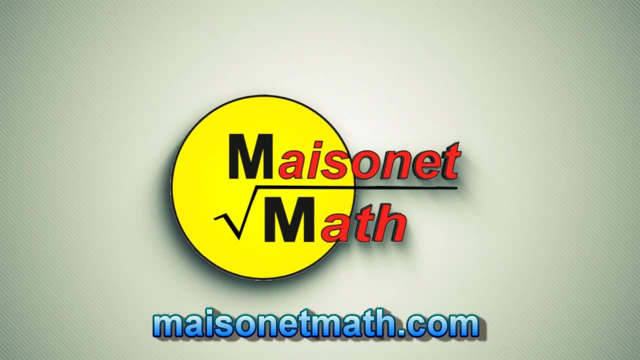 So we are actually able to travel in a given duration of 20 minutes And the whole window of bus route B must have passed. But how many hours? I would say they would have passed by 10 minutes, But let's say 20 minutes. Then the second bus route B would arrive at the same time, 2 hours later. Then the last bus route B would arrive at the same time, 5 minutes later, And so the rule is that the bus route B should have passed by 20 minutes later. And that is what the problem is: That the bus route B should have passed at the time, 20 minutes later, But the first bus route B is not a bus route.